in a graph and trying to find the focus. And we were working on parabolas and, instead of just putting them in a graph and trying to find the focus, and. And we were working on parabolas and instead of just putting them in a graph, and trying to find the focus, and. 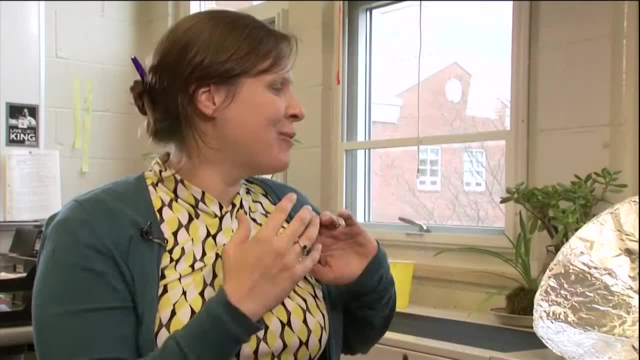 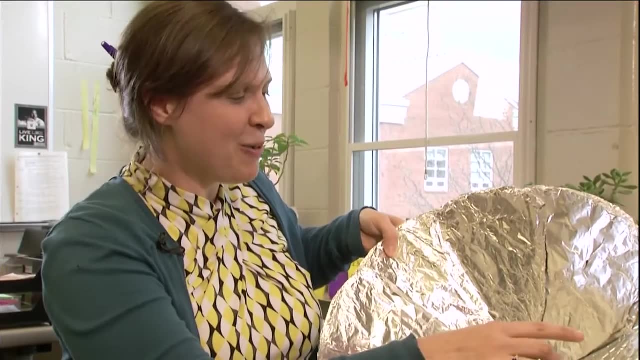 doing all the mathy things we're expected to do in the textbook. we decided that we were going to actually find the focus, because it has this great property that, when the light comes in, it'll hit off of the side of this and it'll bounce into a certain fixed point. 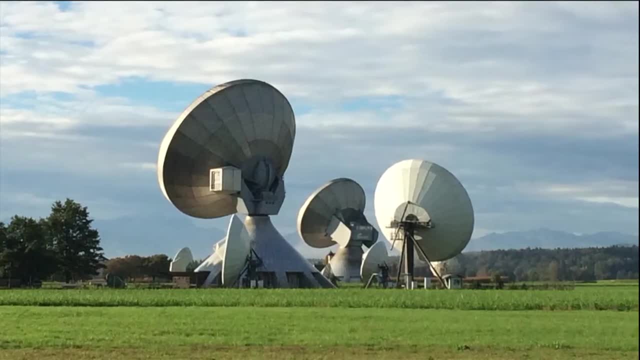 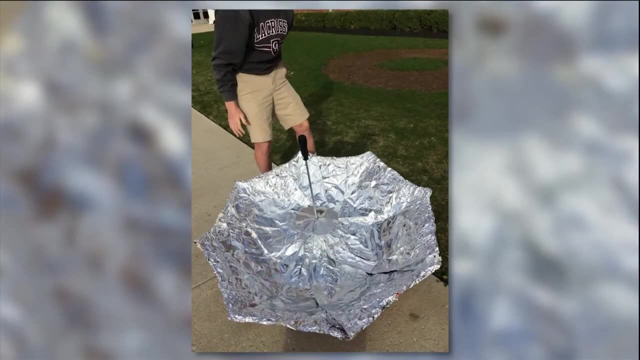